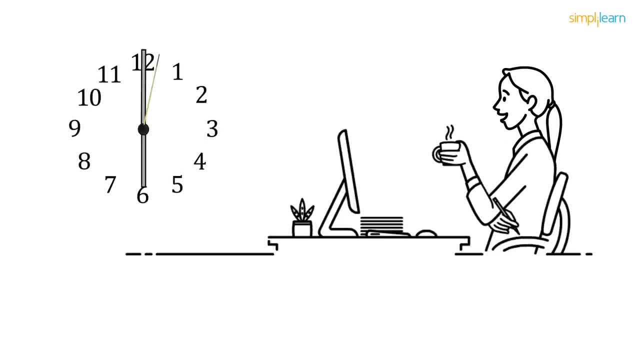 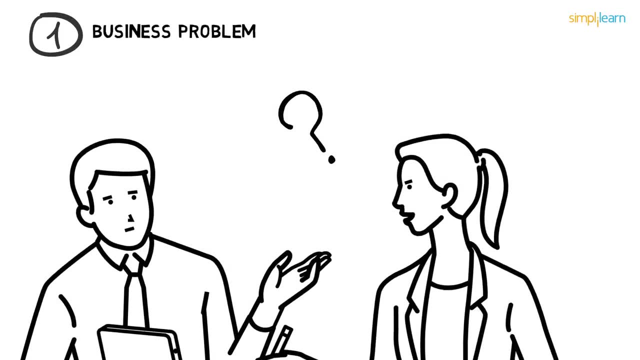 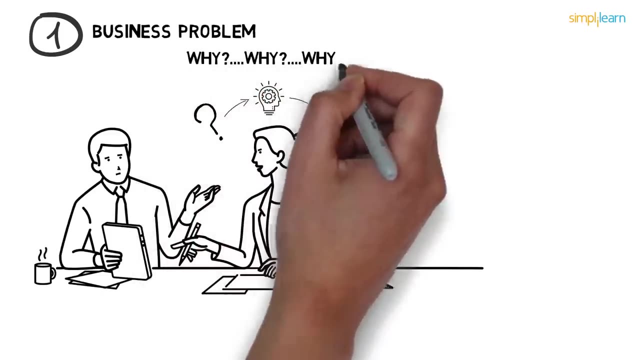 her life goes while she's working on a data science project. Well, it is very important to understand the business problem first. In our meeting with the clients, Emma asks relevant questions, understands and defines objectives for the problem that needs to be tackled. She is a curious soul who asks a lot of buys- one of the many traits of a 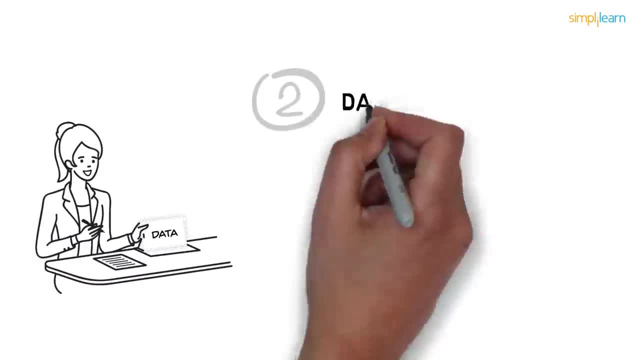 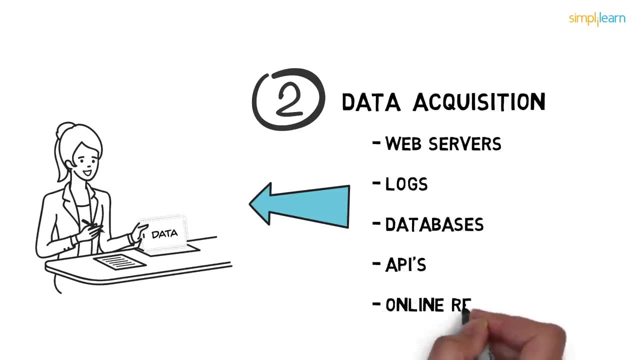 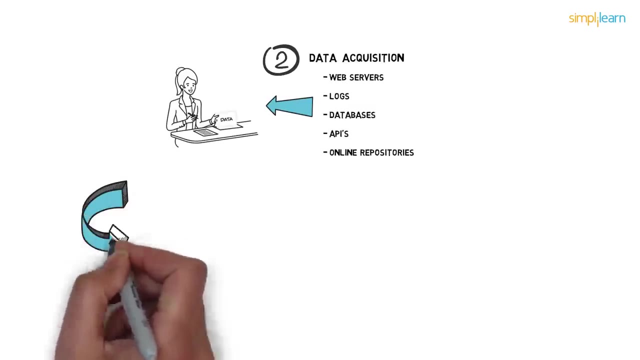 good data scientist. Now she gears up for data acquisition: To gather and scrape data from multiple sources like Web servers, logs, databases, APIs and online repositories. Oh, it seems like finding the right data takes both time and effort. After the data is gathered comes data preparation. This step involves data cleaning. 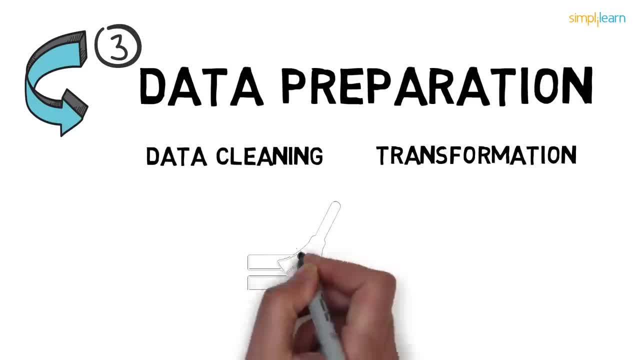 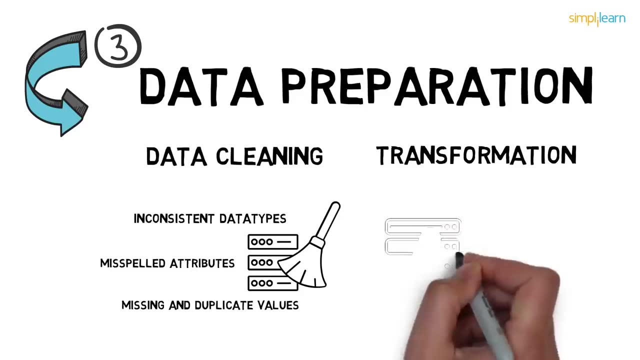 and data transformation. Data cleaning is the most important and the most critical part of your data acquisition. You need to discipline time-consuming process as it involves handling many complex scenarios. here Emma deals with inconsistent data types, misspelled attributes, missing values, duplicate values and whatnot. then in data transformation she modifies the. 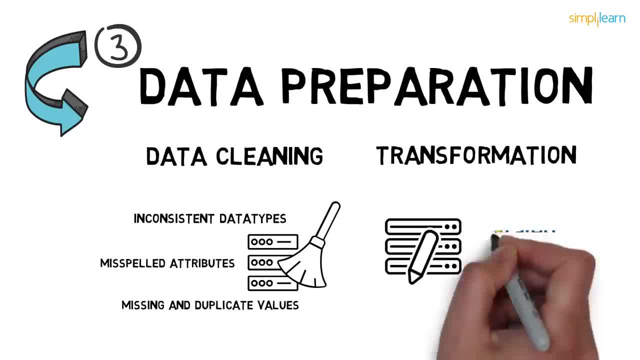 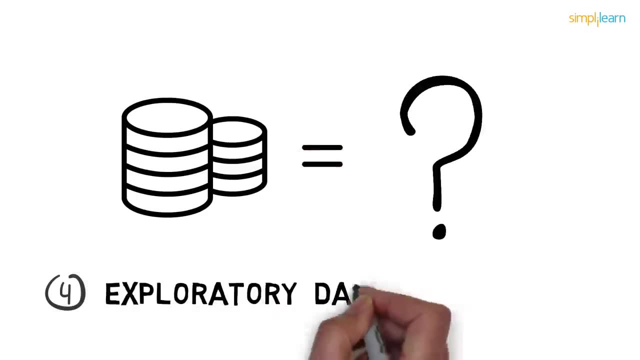 data based on defined mapping tools. in a project, ETL, tools like talent and informatica are used to perform complex transformations. that helps the team to understand the data structure better. then understanding what you actually can do with your data is very crucial. for that, Emma does exploratory data analysis. 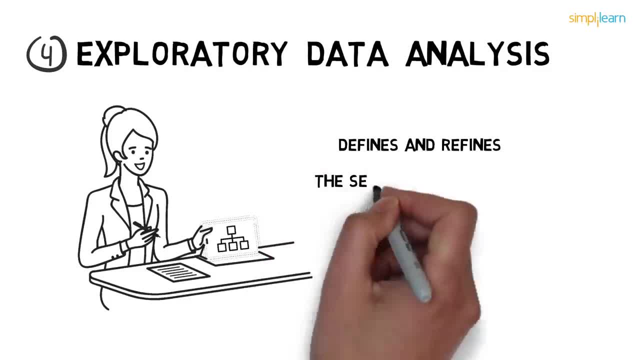 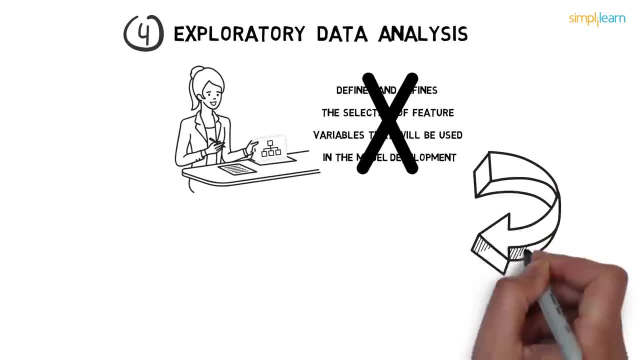 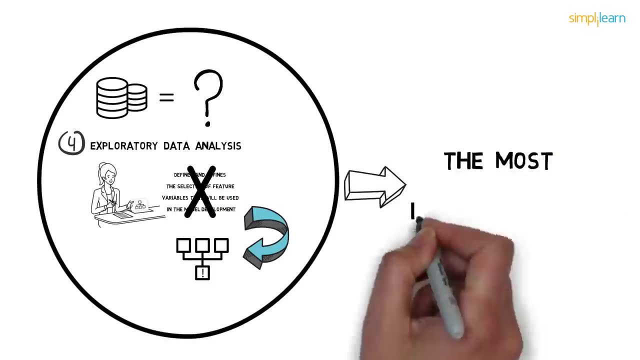 with the help of EDA, she defines and defines the selection of feature variables that will be used in the model development. but what if Emma skips this step? she might end up choosing the wrong variables, which will produce an inaccurate model. thus exploratory data analysis becomes the most important step. 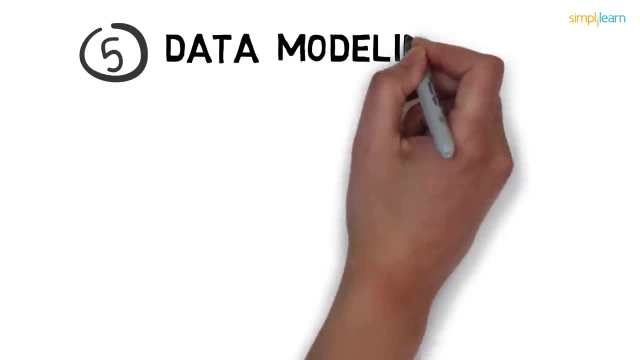 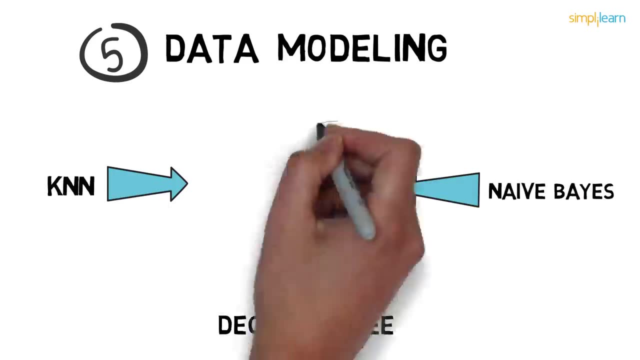 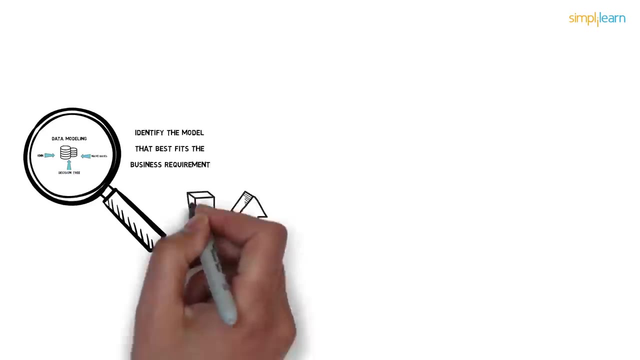 now she proceeds to the core activity of a data science project, which is data modeling. she repetitively applies the data science process to the data science process to identify the model that best fits the business requirement. she trains the models on the training data set and test them to select the best. 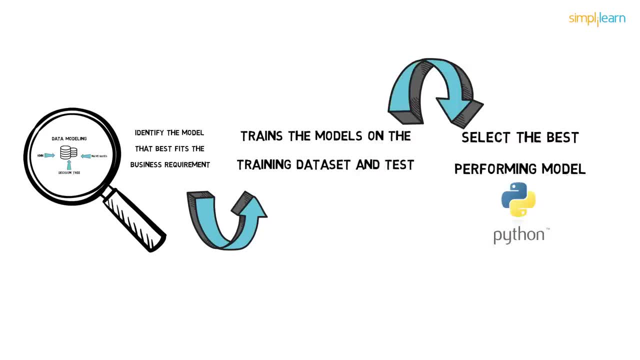 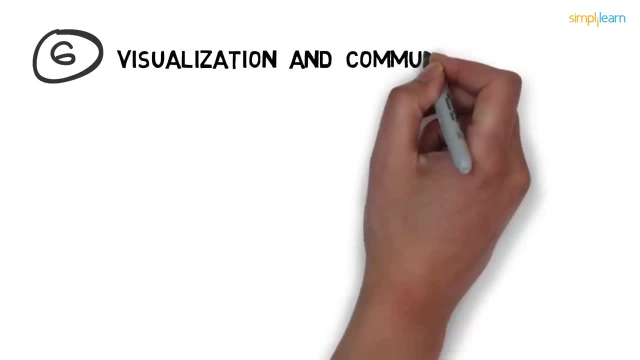 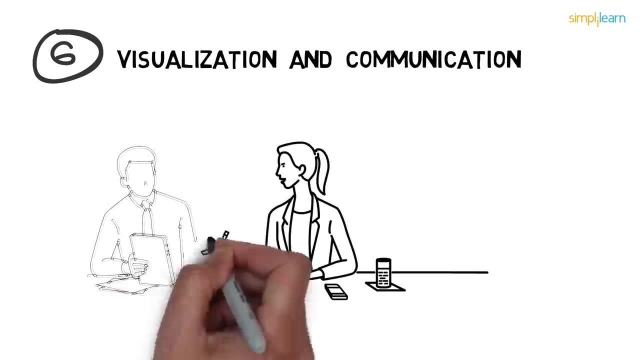 performing model. Emma prefers Python for modeling the data. however, it can also be done using R and SAS. well, the trickiest part is not yet over: visualization and communication. Emma meets the clients again. to communicate business findings in a simple and effective manner. to convince the stakeholders, she uses tools. 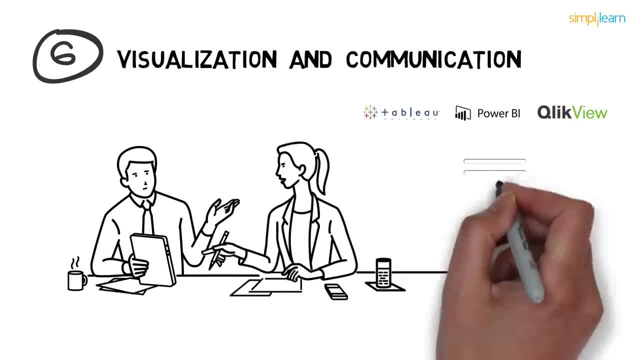 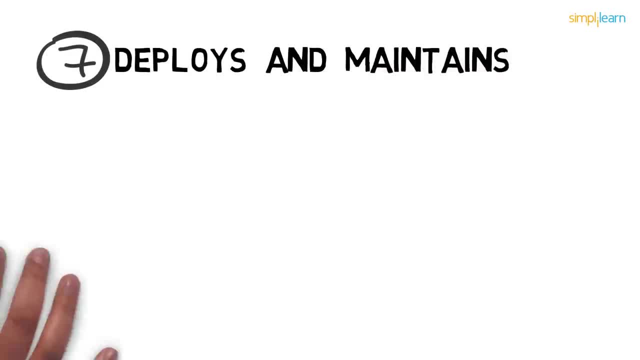 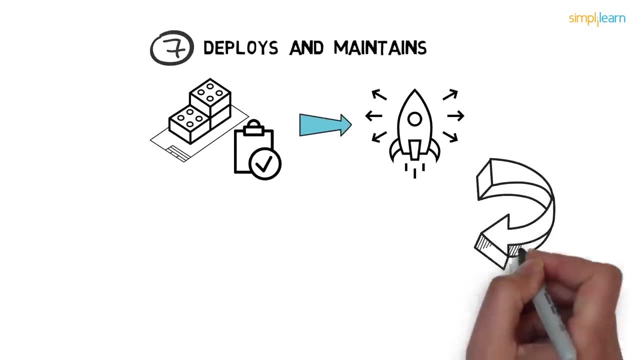 like tableau, power bi and click view that can help her in creating powerful reports and dashboards. and then, finally, she deploys and maintains the model. she tests the selected model in a pre-production environment before deploying it in the production environment, which is the best practice. right after successfully deploying it, she uses reports and dashboards to get. 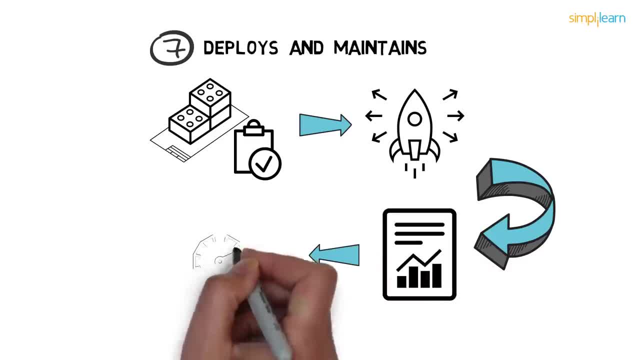 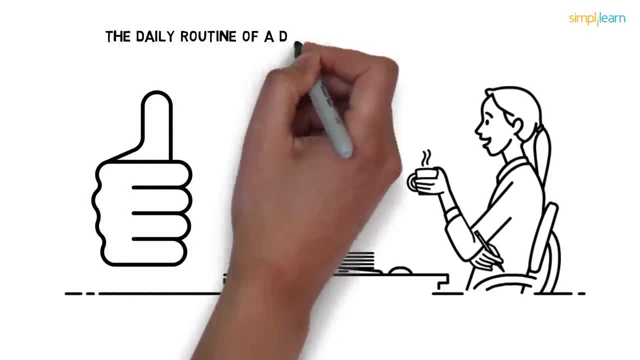 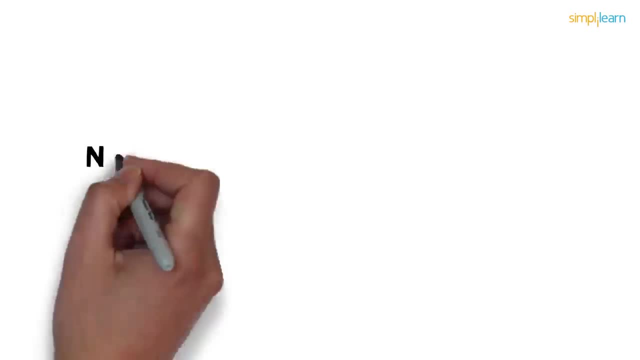 real-time analytics. further, she also monitors and maintains the projects performance. well, that's how Emma completes the data science project we have seen. the daily routine of a data scientist is a whole lot of fun, has a lot of interesting aspects and comes with its own share of challenges. now let's see how data science is changing. 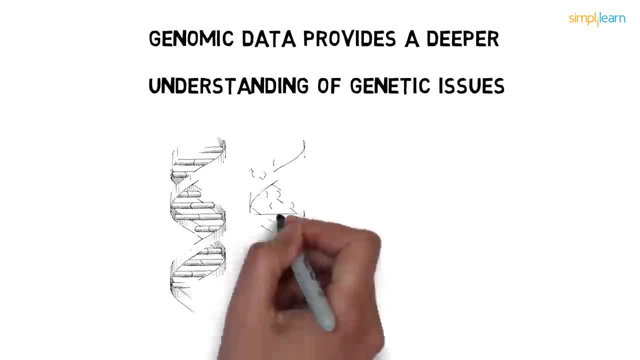 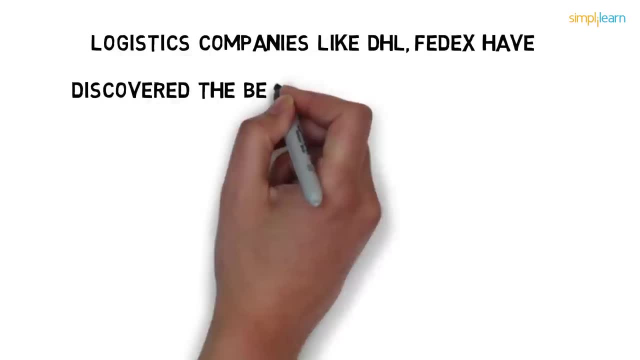 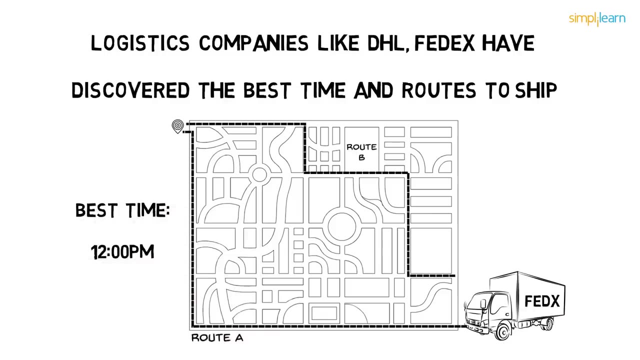 the world. data science techniques, along with genomic data, provides a deeper understanding of genetic issues in reaction to particular drugs and diseases. logistic companies like DHL, FedEx have discovered the best routes to ship, the best suited time to deliver, the best mode of transport to choose, thus leading to cost efficiency with data. 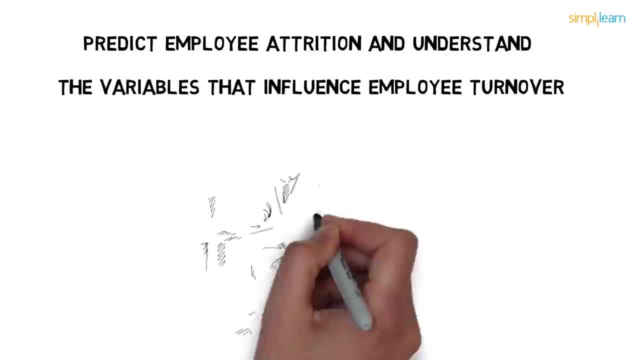 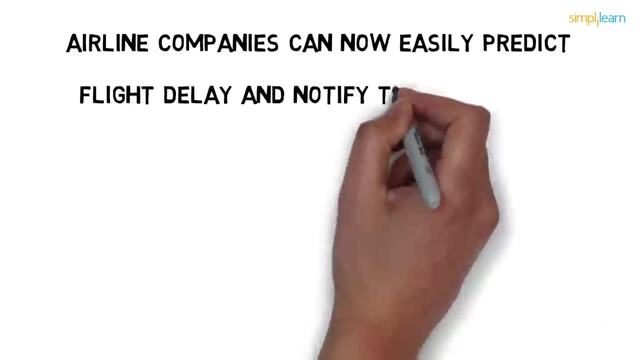 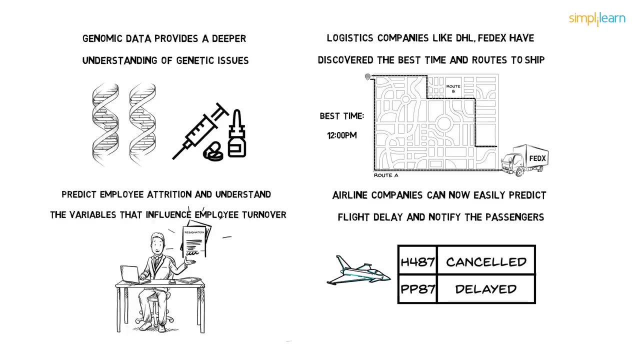 science, it is possible to not only predict employee attrition, but to also understand the key variables that influence employee turnover. also, the airline companies can now easily predict flight delay and notify the passengers beforehand to enhance their travel experience. well, if you're wondering, the various rules are hit and run. so far, we're on a long way to getting the data science team to understand what's going on and how it's going to impact their business today and how it's going to affect their business then. we'll talk to them in the next few minutes. 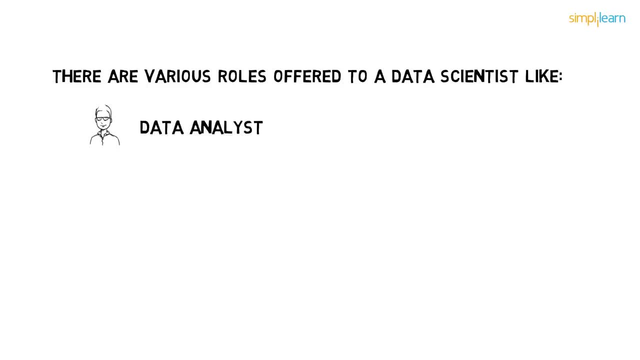 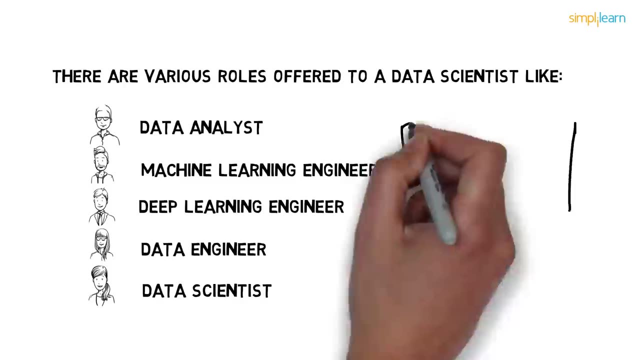 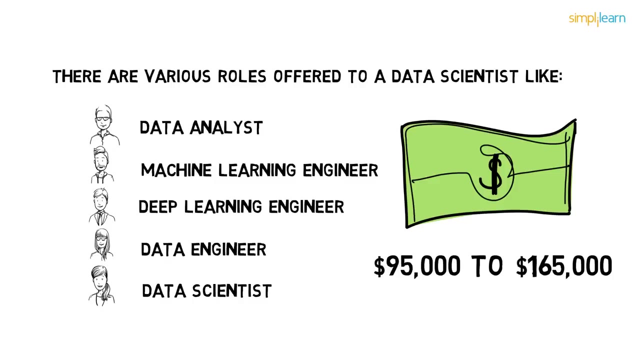 offer to a data scientist like data analyst, machine learning engineer, deep learning engineer, data engineer and, of course, data scientist. the median base salaries of a data scientist can range from $95,000 to $165,000. so that was about the data science. are you ready to be a data scientist? if yes, then start. 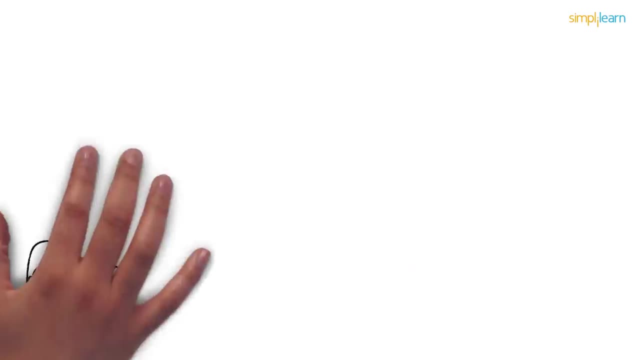 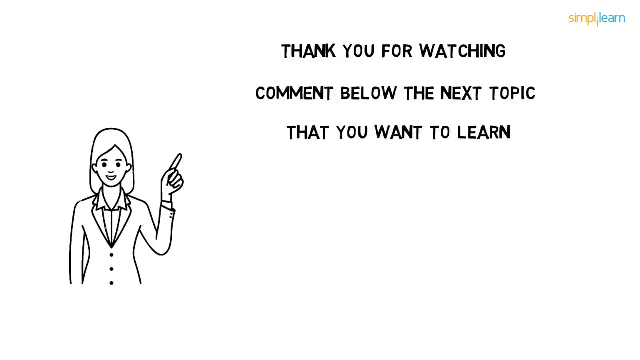 today, the world of data needs you. that's all from my side today. thank you for watching comment below the next topic that you want to learn and subscribe to simply learn to get the latest updates on more such interesting videos. thank you, and keep learning.